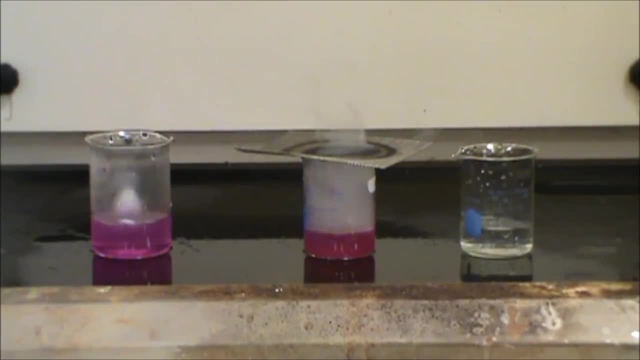 So you'll see some orange flame perhaps, or some sparks, or some shrapnel. And then the last one. I'm going to go ahead and put my two pieces of potassium in that I've cut in half, So this is less potassium than the other two in terms of amount. 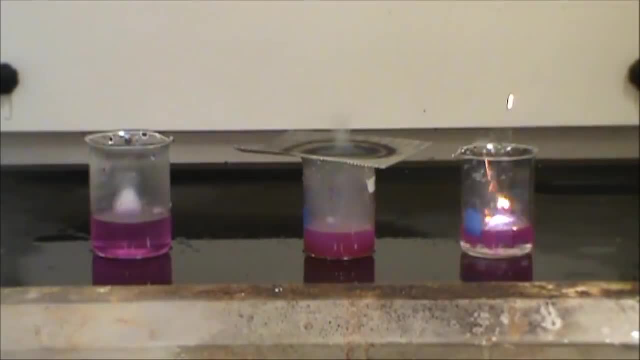 but I'm going to add more potassium. What AM ga does is it can ignite, lit the potbelly and you'll see a little of that in as little as, say, six or seven figures due to quantization. Look, we're going to just put all this in. 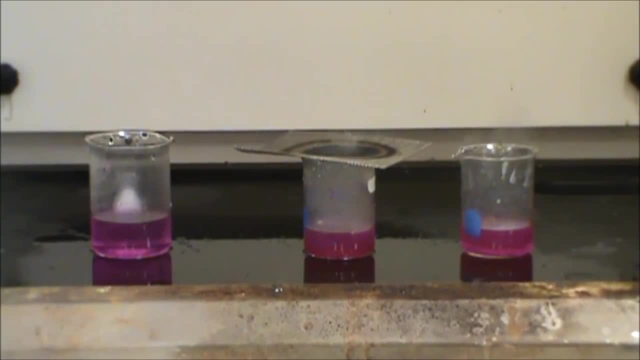 If we put all of this in two we can see the push and pull of the potassium. if one が, as I will show in the link, that just gone up and out of the prairie water, is going to start getting a little more about industriallyier if we just give it, got our. 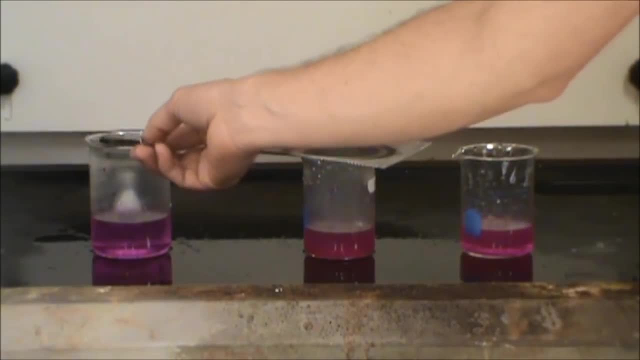 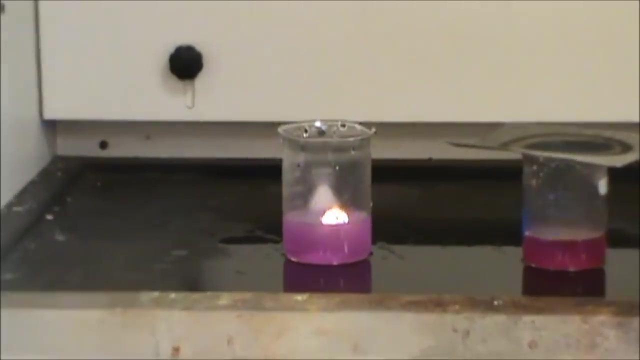 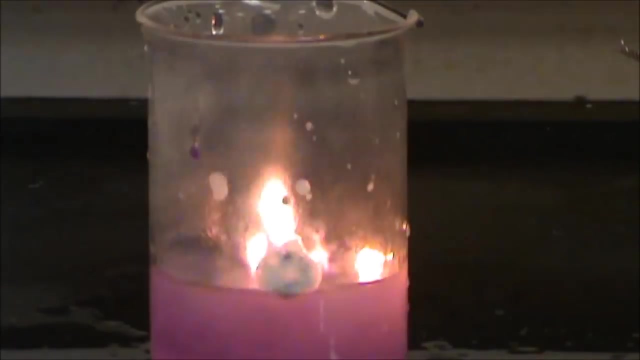 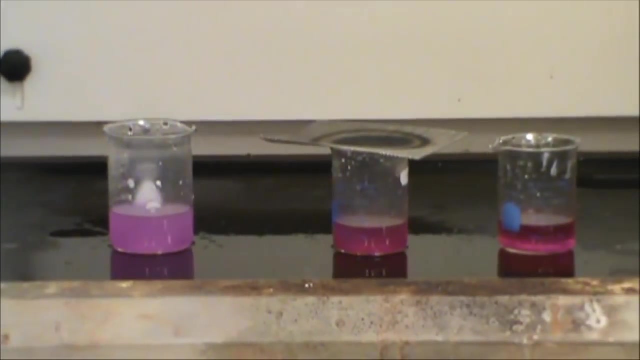 마지막 dose of potassium. Okay, See, can try adding another piece here. We can hope that that's going to go ahead and actually send off some shrapnel and some flame. All three produce hydrogen gas, all three produce hydroxides. and there's your. 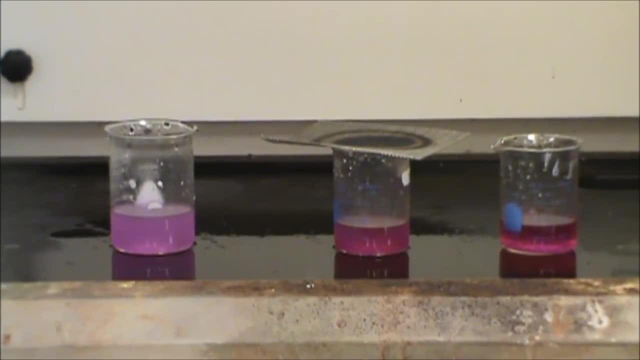 alkali metals. Next we're going to go ahead and do the rubidium and cesium. 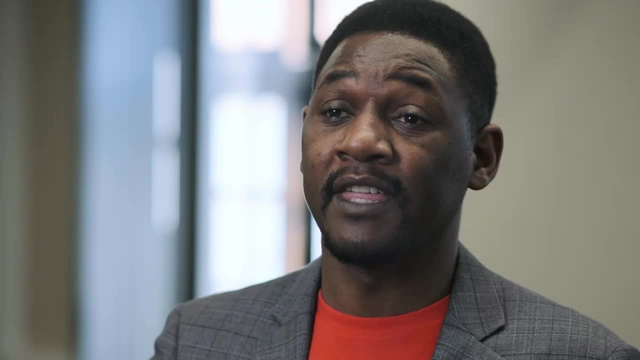 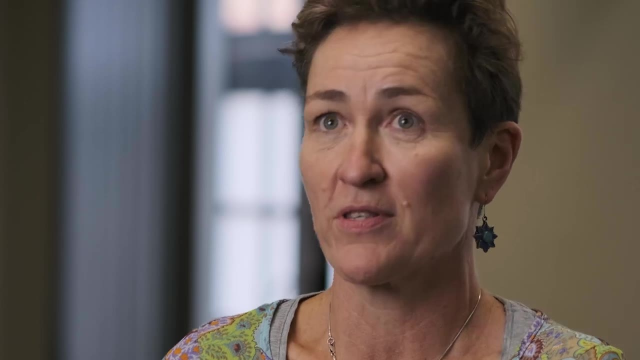 Climate resilience is a really difficult term. It means different things to different people. Some people could describe it as a very slippery term. It feels intuitive that you should know what it means and it sounds positive. If you don't define it clearly then it's very difficult to 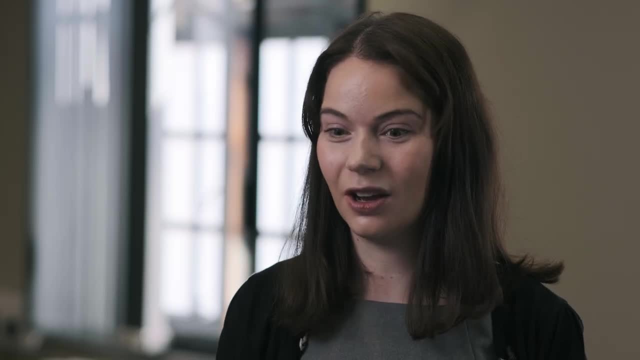 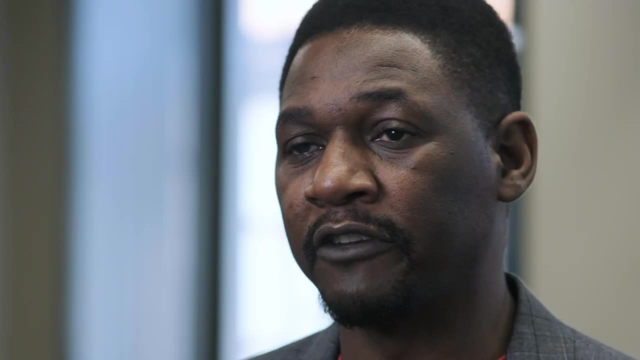 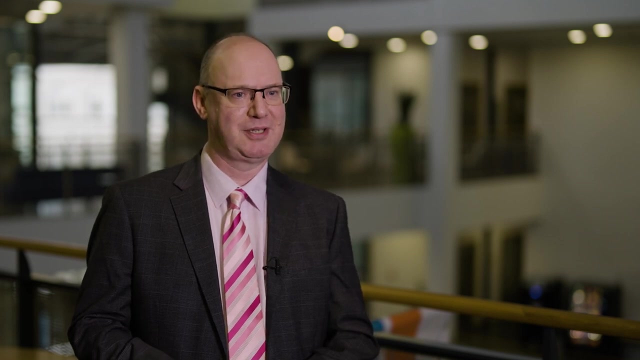 put into practice. Personally, for me, climate resilience is all about ensuring our people and places are adapting and prepared for our changing climate. We might be finding new ways of managing climate risk. all together, It's really about how we cope with the challenges of climate change, how we exploit any benefits that come with climate change.